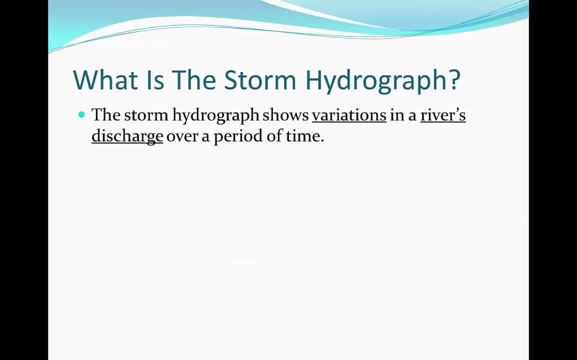 in a river's discharge level over a period of time. Now the word discharge is a term used to describe the volume of water that passes through a river at a given moment in time, So this tells us how much water there is in the drainage basin system and also the potential it has to then. 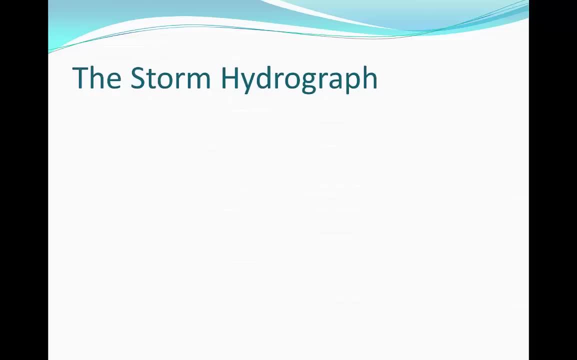 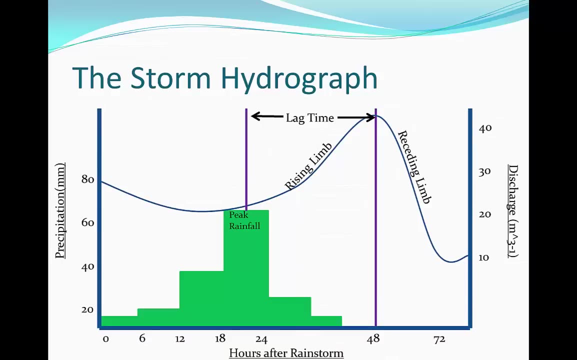 overflow. So how do we draw the storm hydrograph On screen? now is the storm hydrograph. Now it may seem weird to you at first because there's three sets of axes, but we need this to show three different variables. So on our x-axis, running along the bottom, we have the hours after a rainstorm. 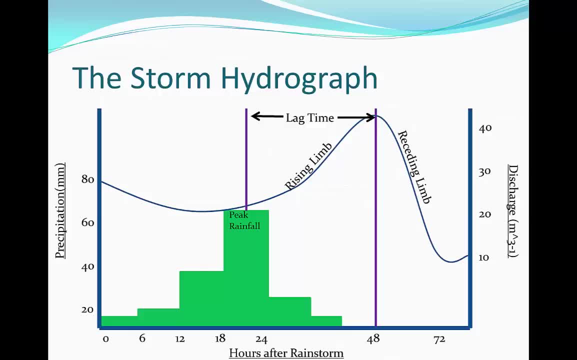 on our y-axis on the left, we have precipitation levels in millimetres, and our y-axis on the right shows levels of rainfall. So what I would like to do now is pause the video and have a go at copying this down and, whenever you're ready, hit place when we can then describe. 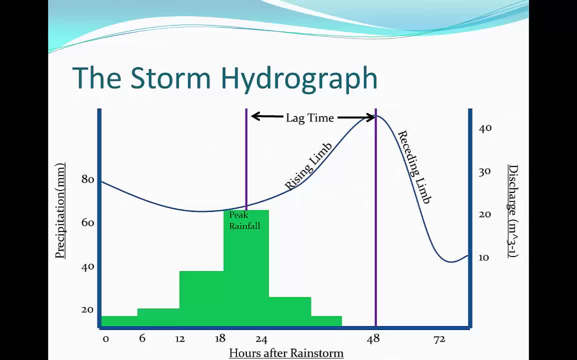 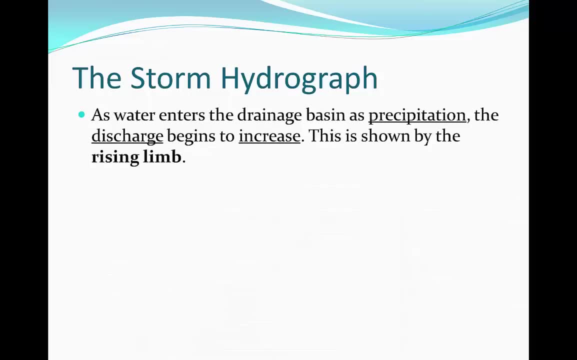 and explain the processes of the storm hydrograph in more detail. Okay, so the first thing that the storm hydrograph is going to show is its levels of precipitation. So, as we can see on the graph now, the precipitation is shown by the bars. 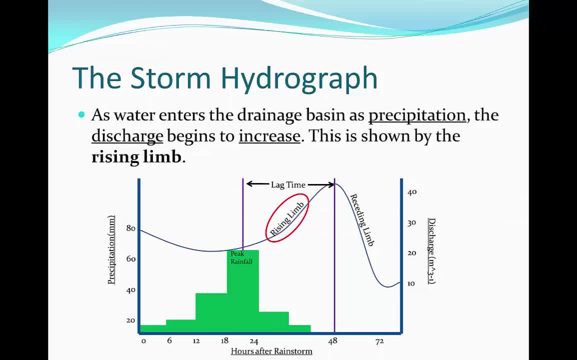 so these green little bars that come up on the left hand side of the graph. So what this shows is that when there is a rainstorm, generally levels of precipitation start quite low, under 20 millimetres, between the first zero and six hours. Then, as time goes on, there begins to. 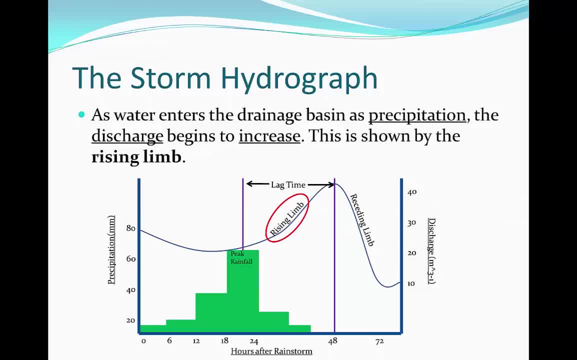 accumulate more and more rain, and it generally rises until the 24-hour period where we reach peak rainfall. As this happens, the rising limb is going to increase, and what the rising limb shows is that the increase in levels of discharge. So you may be thinking to yourself. it seems weird. 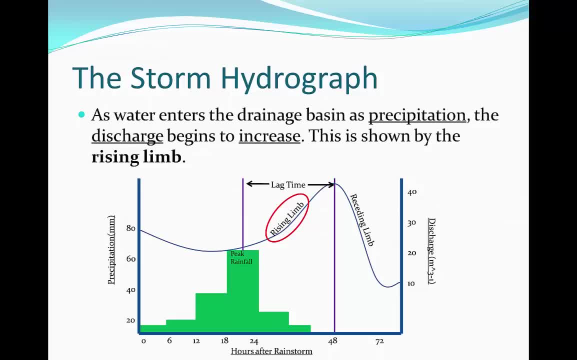 precipitation increases, discharge in fact decreases in the early hours after the rainstorm. So between 0 and 18 hours it seems that discharge is decreasing. So why is it that when precipitation increases, discharge decreases, And this is down to the lag time. So what the lag time really shows is the time 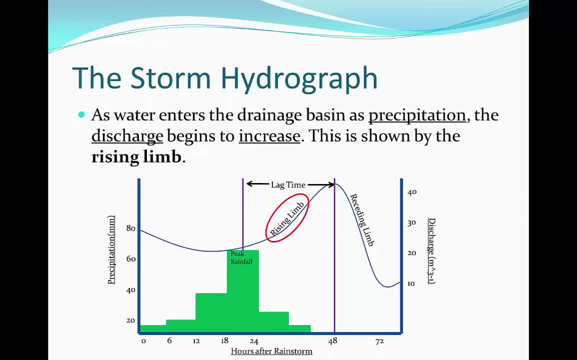 it takes between peak rainfall and peak discharge. As it begins to rain, a lot of that rain falls into the soil of the river. Now, this saturates the soil as the pores up with water. as a result, the discharge isn't increasing at all, because the river is just